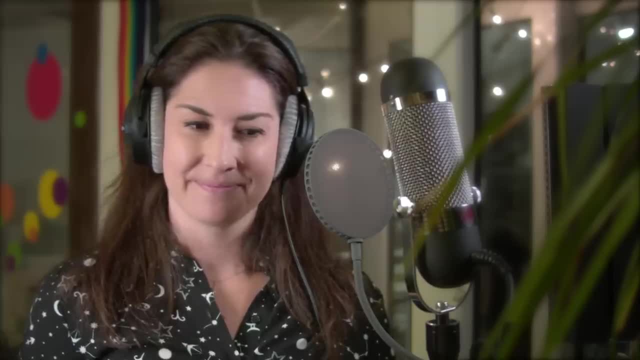 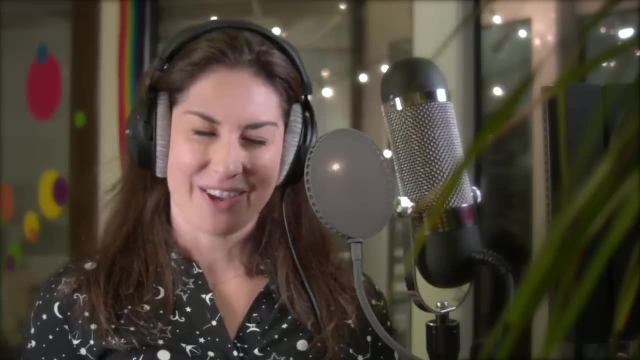 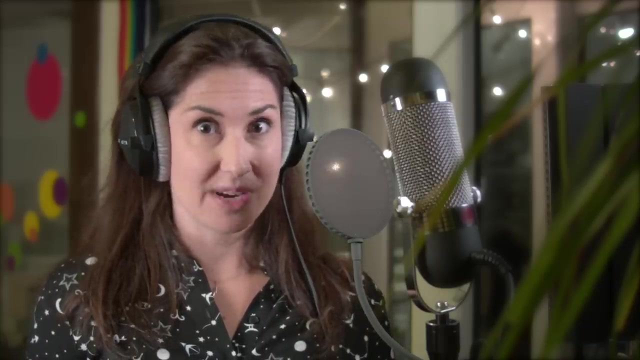 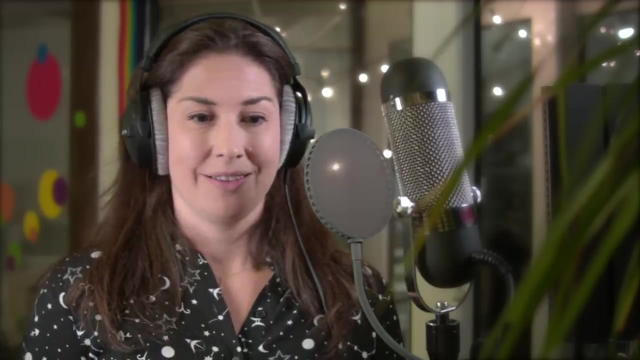 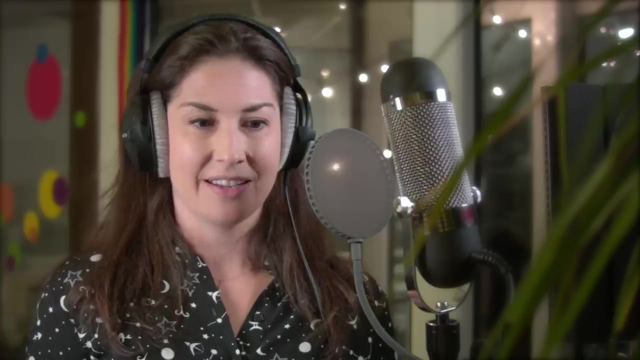 allow your body to settle. Okay, now you're settled And you're in a good spot. Let's listen to our breathing. It might be very quiet- quieter than a whisper- But if you listen carefully, you might just start to hear it Coming in. 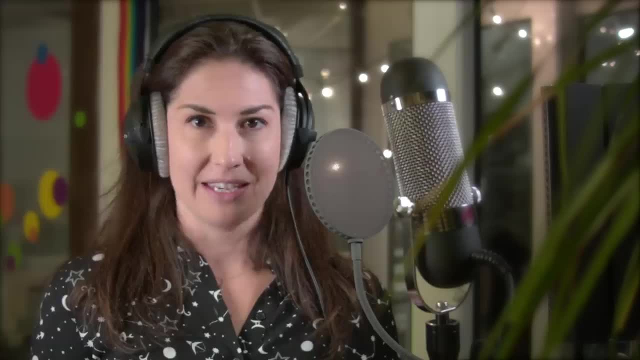 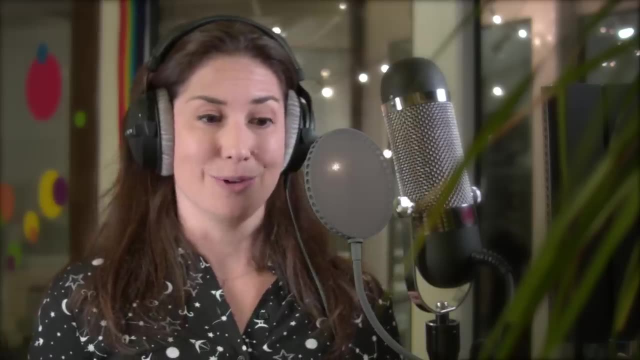 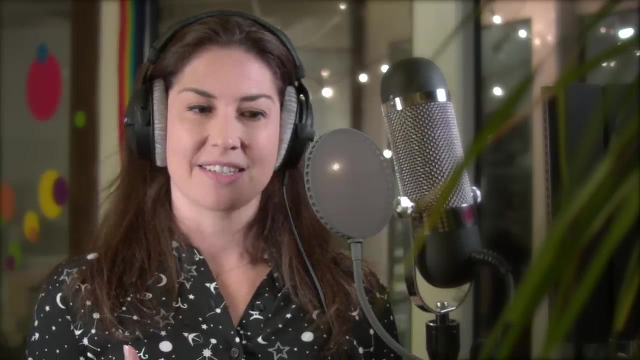 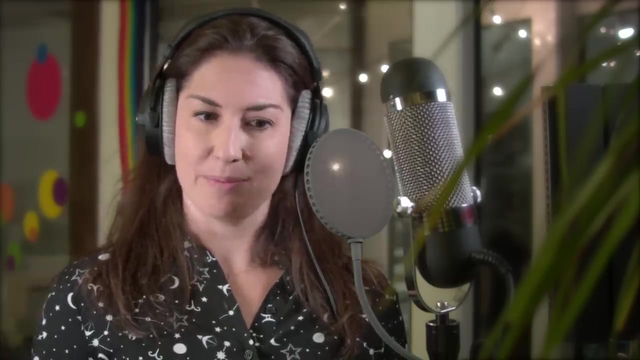 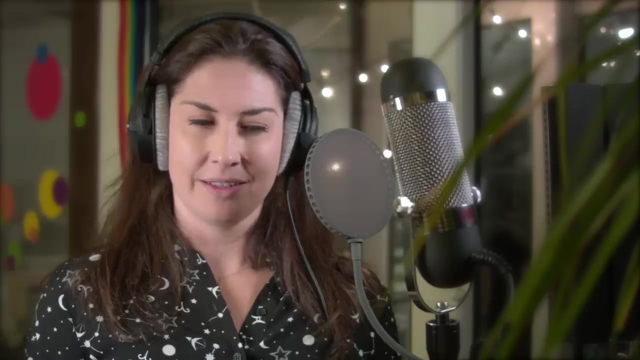 and going out. Coming in and going out. Maybe you can feel it too Around your nostrils as the air comes in and out Your chest, lifting and lowering Even your tummy as it fills up and empties with each breath like a balloon. 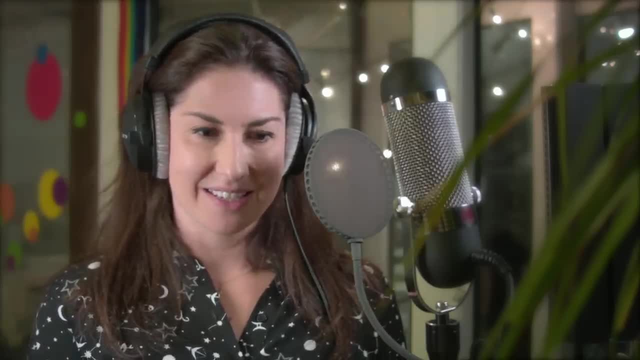 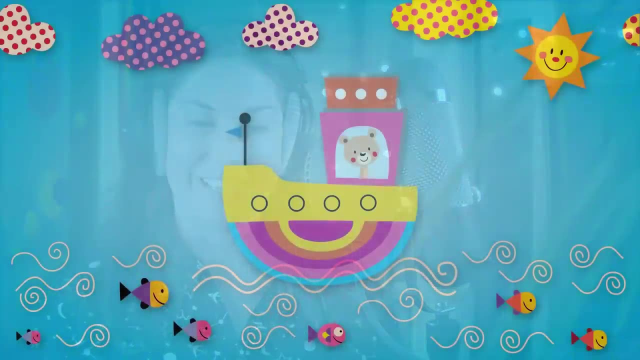 If you haven't already. just allow your eyes to gently close. Now you're in your mind And you can enjoy being taken on a lovely, dreamy adventure. You are at the ocean, Standing on a beach, The sun is warm And there's a little breeze. 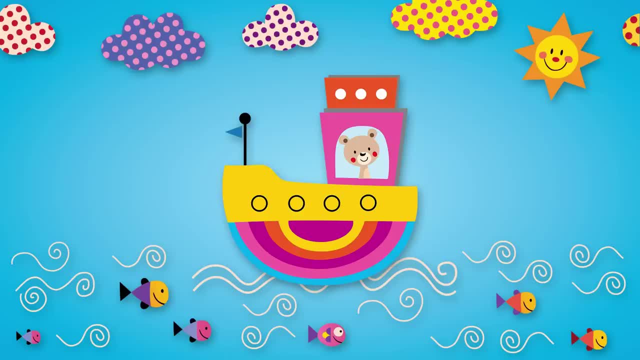 which you can feel on your body and face. Sitting by the water's edge, You can feel the peace and chaos, the floor, Sache, Feeling the aromatic air. Nose, Orleans, Montreal, See you bye, I'm running outta here. 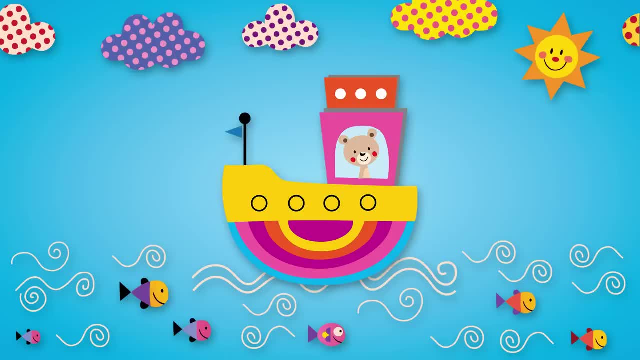 Sался's. This boat is for you. So you untie the rope and give it a push, Hoping in. once you get deep enough, Off you go, Being carried by the waves out to sea. What a lovely feeling. this is Freedom. 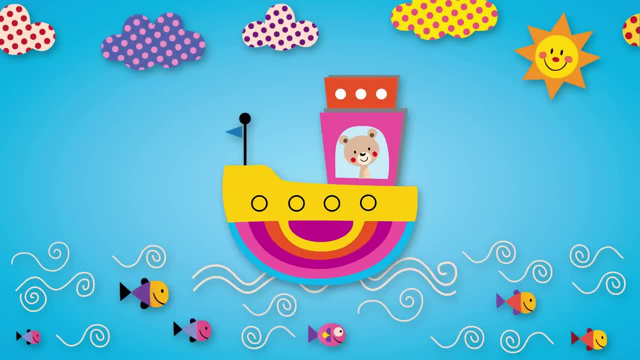 on the ocean. The sun feels warm on your face and body. Yes, Runya, 00.03, Mystery 00.09. What a lovely feeling. that is freedom on the ocean. The ocean waves gently rocking you. It's peaceful here at sea. 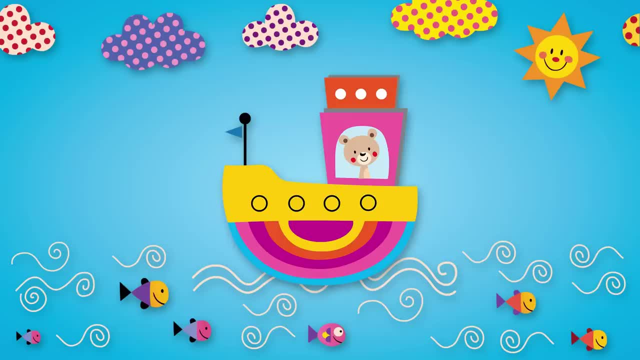 Just the sound of the birds, above and far away, Little splashing sounds of water as the waves meet the boat In the distance. you pick up on another sound, A humming noise. It's very quiet to begin with but gets louder and clearer as it comes nearer to you. 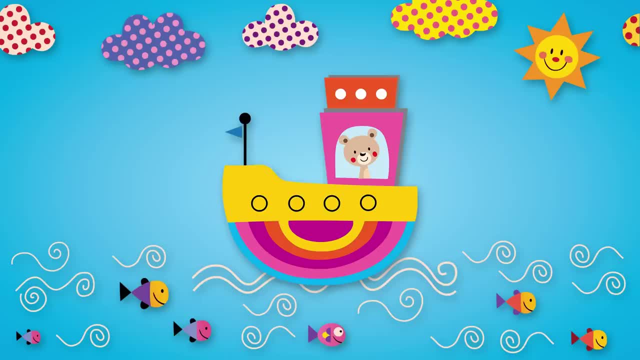 You recognise the sound as another boat. The driver is a kind old man. He is smiling peacefully as he pulls up next to your boat, He turns the engine off and tells you he has brought the bye-bye boat for you. He then asks for your worries. 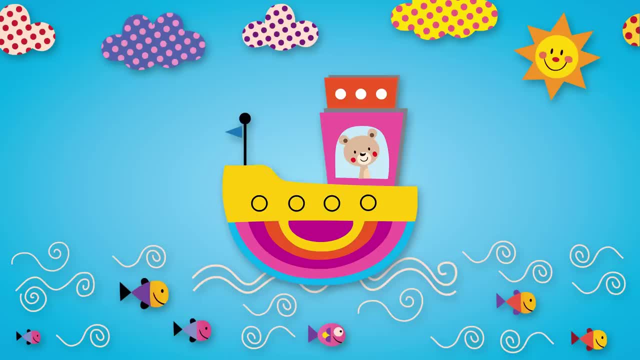 He wants you to hand them over to him. You take a moment to think of all your worries, Every last one. You pack them up and pass them over, putting them onto the bye-bye boat. Next, the kind old man Asks for your anger. 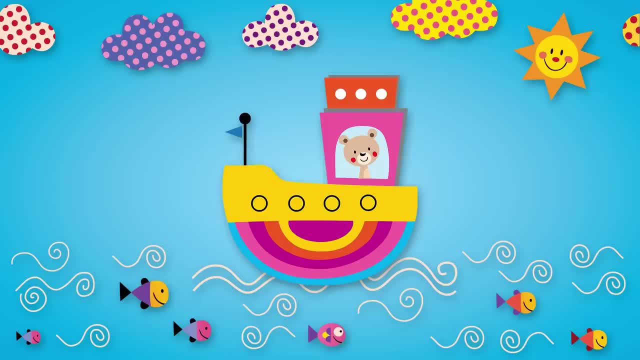 Again, he'd like you to put it on the bye-bye boat. So you get all of your anger, Everything that's really frustrating. You gather it all up and you do just that: You put it onto the bye-bye boat. 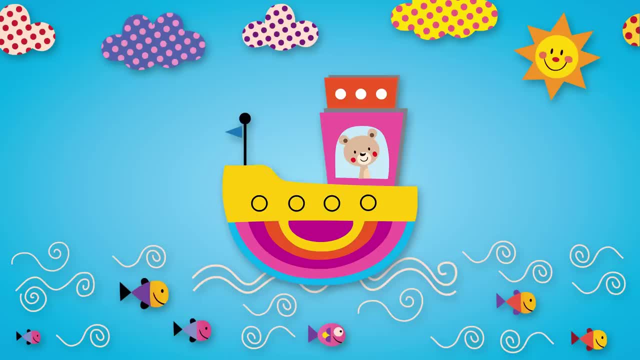 Finally, the kind old man Asks for your fear. You make a special effort to collect all of your fear, All that. you are afraid of Every last bit of it, And you hand it over, putting that on the bye-bye boat as well. 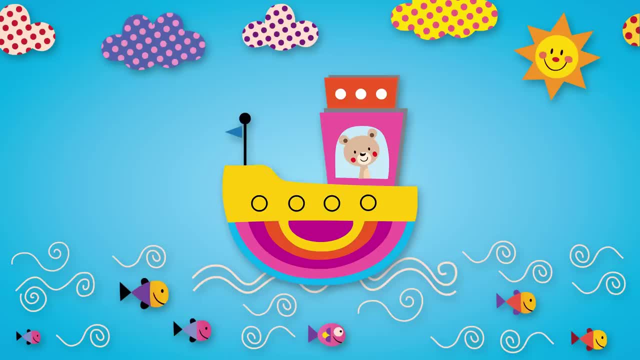 The old man looks and smiles at you. You smile back at him enjoying the moment. You feel so good now. You feel light. You don't have any worries, anger or fear to carry anymore. You are free. The old man starts the engine.